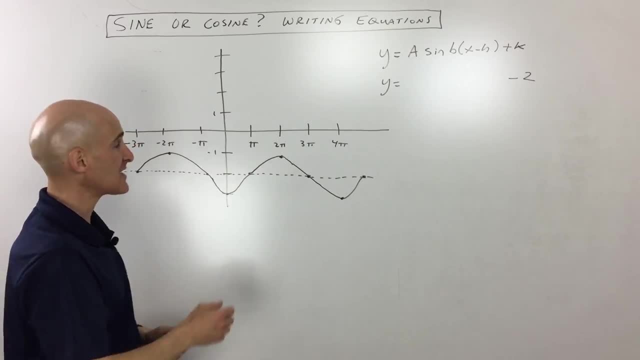 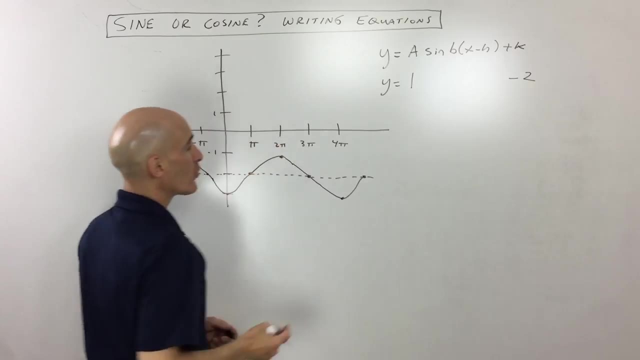 positive. If it's negative, what that means? it's reflecting it over the x-axis. So you can see this amplitude here is just a height of one, And if it's negative it's reflecting it over the one one. So we know our a value is one. Now the question is: do we want to use a sine graph or a? 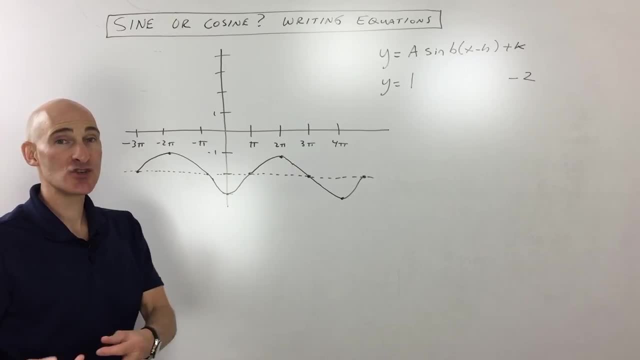 cosine graph. Well, again, that has to do with what you want to think of as your starting point. You want to know your basic sine and cosine graphs, So I'm just going to sketch them right here so you can see this Sine normally we think of as starting here, at the origin, and then it. 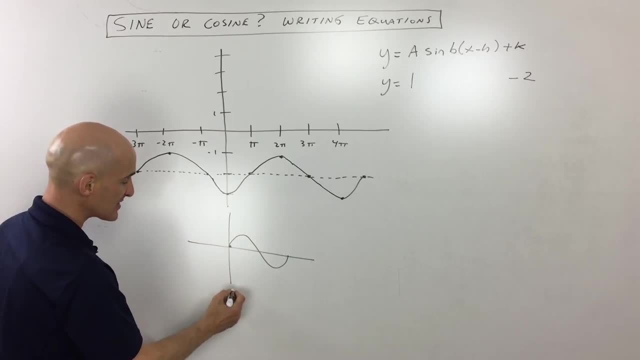 goes up and then back to zero and down and back up, like that, right? So that's the basic sine graph, Whereas a cosine graph starts at the maximum, goes through the minimum, back to the maximum, like that. They both have a period of two pi And what we want to do is: 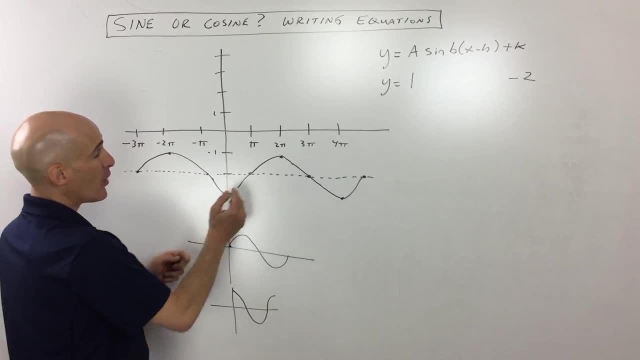 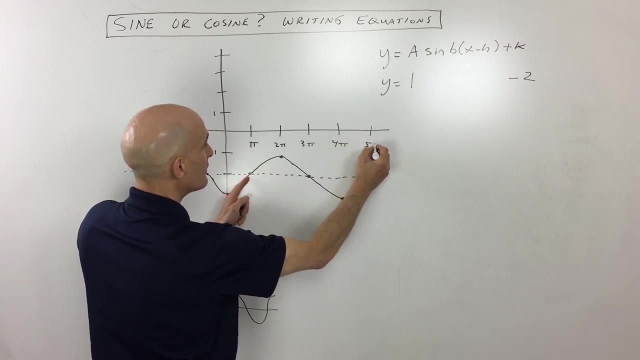 we want to calculate what the period is for this particular graph. Now, to get from, let's say, this point to where? then it starts over and repeats again. that's giving us a distance of four pi. okay, Five pi minus one pi, four pi until it repeats. The other way to do it is you. 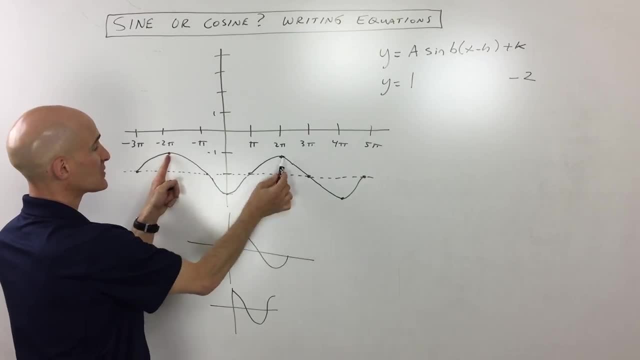 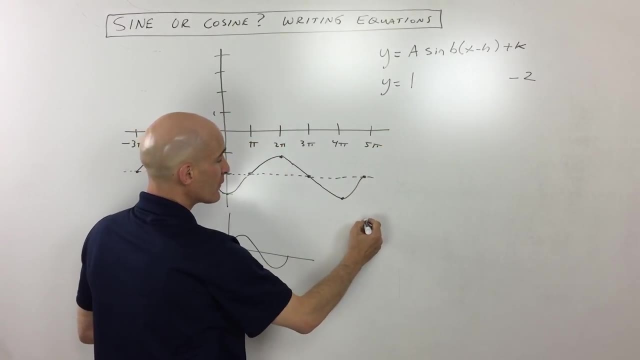 can measure from peak to peak or from valley to valley. So this is still giving us four pi. This is still giving us four pi. So in this case, let's go ahead and calculate with this b-value. So we're going to calculate what the b-value is, And the formula for this is: the period is equal to two pi. 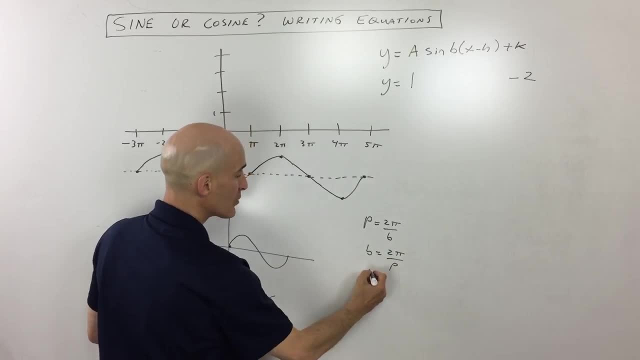 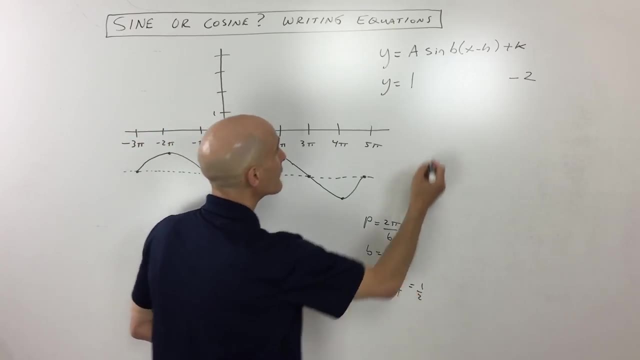 divided by b. or you could say b is equal to two pi divided by the period. In this case, the period we set is four pi. So if we reduce you can see that b is equal to one half. So in any of these, 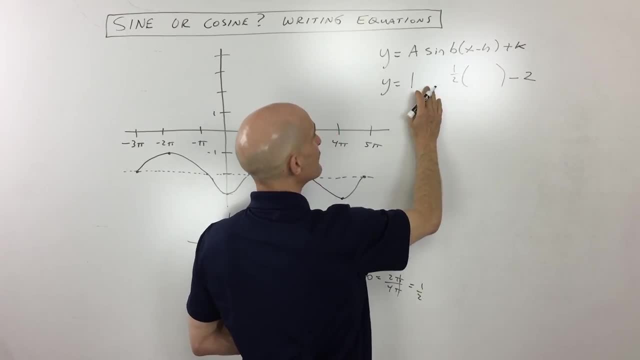 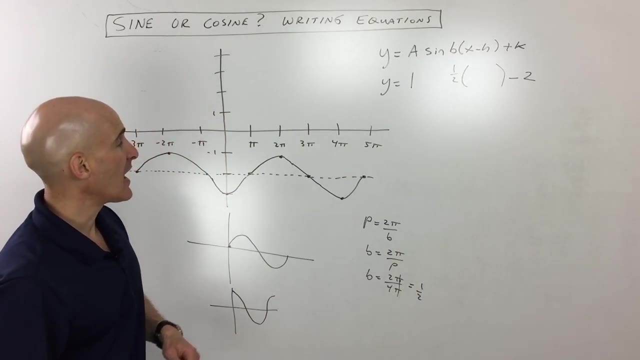 equations that we're going to be writing here. we're going to have the same basic format. We're going to have: amplitude is one, b is one half, the vertical shift is negative two. But then what we want to analyze is: okay, are we going to use a sine or a cosine? Are we going to use a sine or a cosine? 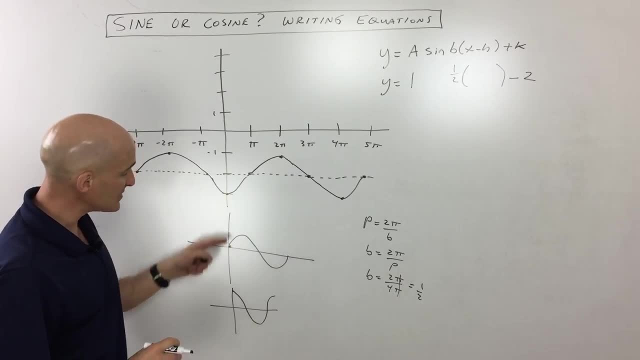 Let's maybe start with a cosine graph Now. you see this cosine graph down here. If I was to reflect it over the x-axis, then it would be over here, right, And it would look something like this dotted line that I'm drawing right now, which looks a lot like the graph that we have here, right. So I'm 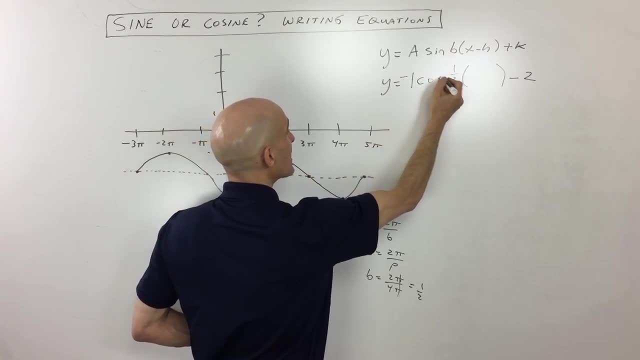 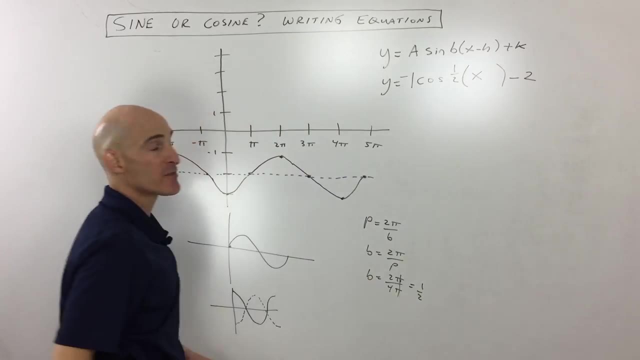 going to make this a negative one. cosine one half x. okay, Now it hasn't shifted left or right, so my h-value is just going to be zero. I'm just going to leave it like that. The only thing that's differing between all these equations that are going to be here is that I'm going to have a. 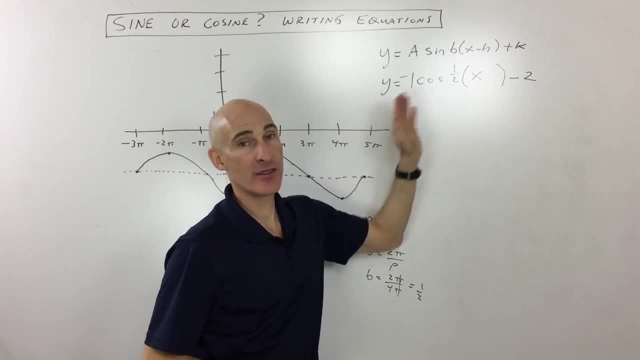 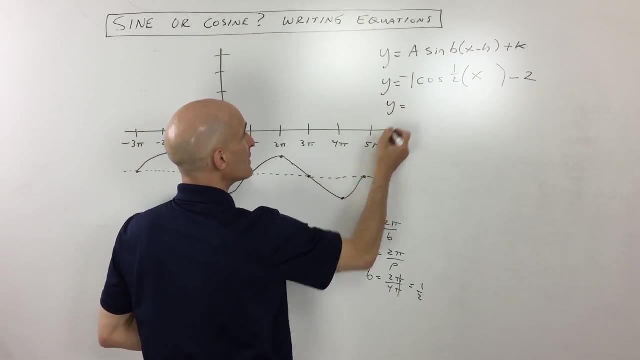 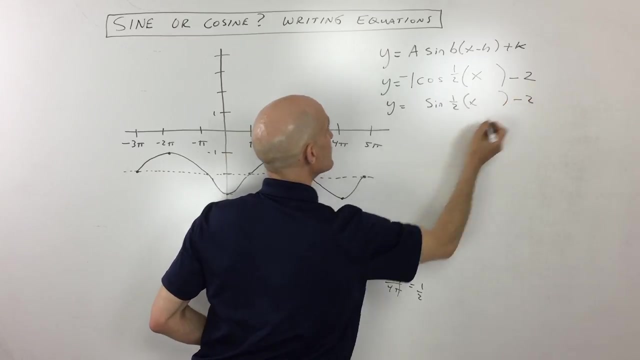 positive or negative, and the phase shift, which is the left and right, the horizontal shift. Okay, so that's one possible answer here, right? The next one is: let's maybe take a sine graph now. So we're going to say sine. we still have the one half, we still have the negative two. Now remember, 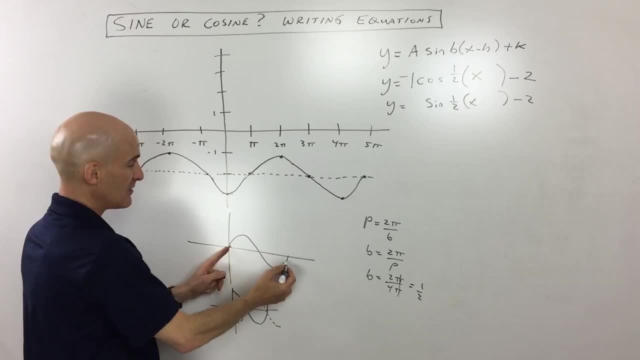 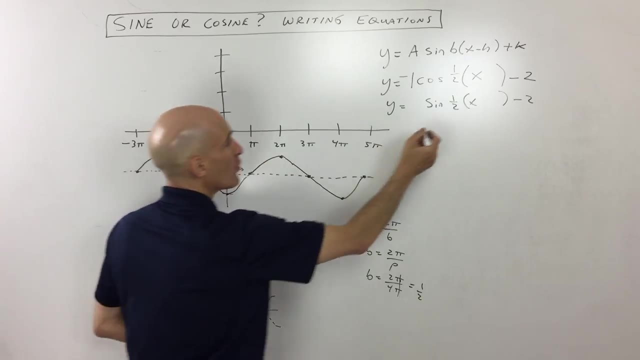 sine starts here, at the origin, and it goes up and then down and back up. So you can see, this would be like a starting point, but what's happening is it's shifting to the right pi. So when we shift to the right, that's going to be minus pi. Remember, the one that's grouped with the x has. 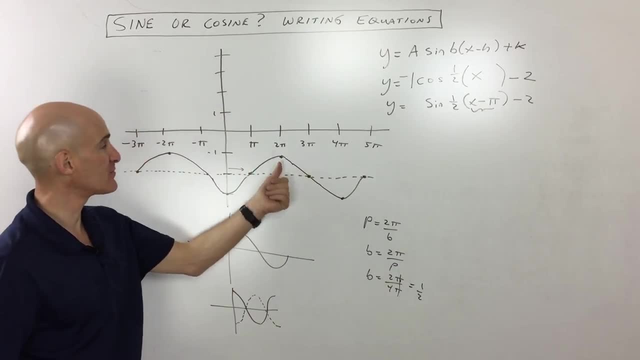 the opposite effect on the graph: Minus pi is actually shifting right pi. plus pi is shifting left pi. okay, And then the other question is: is that, has it been reflected or not? Well, this one hasn't been reflected. You can see. it's the same shape as this graph here. It's just being shifted. 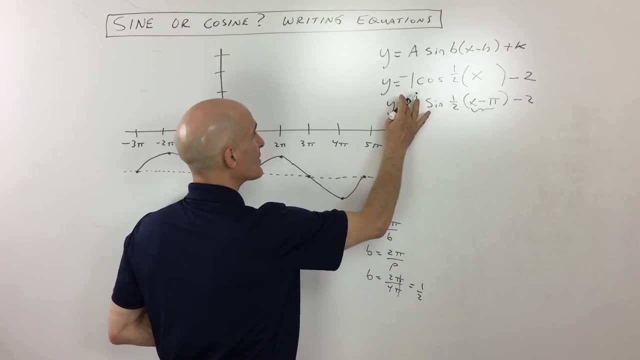 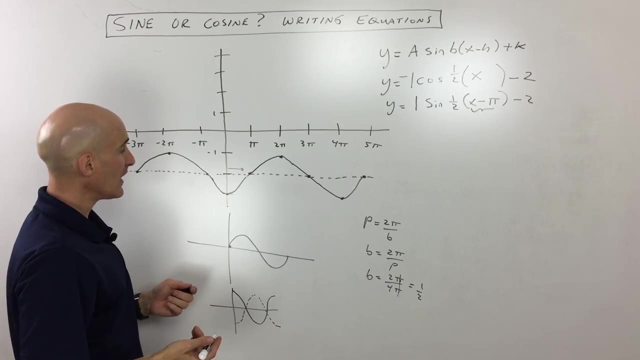 right. So that means the amplitude is just going to be one. It's not going to be multiplied by a negative. Okay, let's take a look at another example. Let's maybe say, for example: we want to do a sine graph, but we want to make a sine graph. So we're going to do a sine graph, but we want to make a. 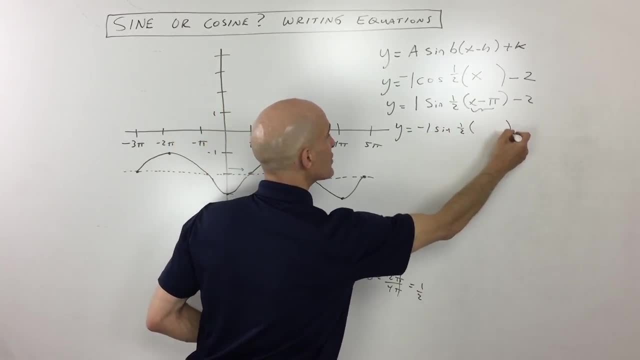 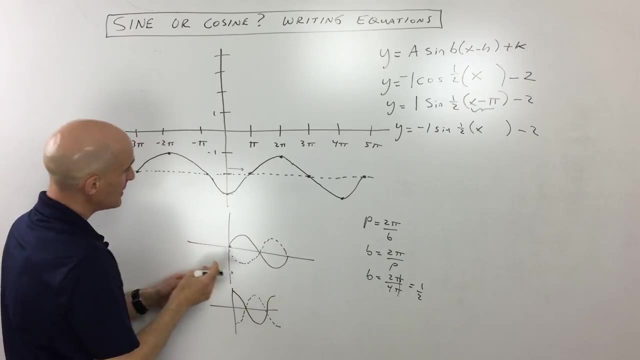 negative amplitude this time. Okay, so all this information here is staying the same. The only thing that's changing is the fact that this is going to be a negative, so it's reflecting over the x-axis. So where does that look like? Well, that looks something like it's starting here now. 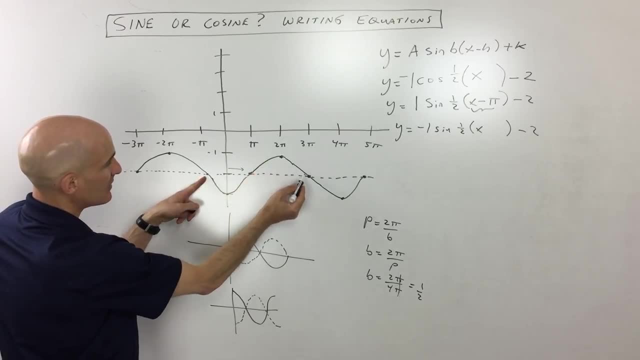 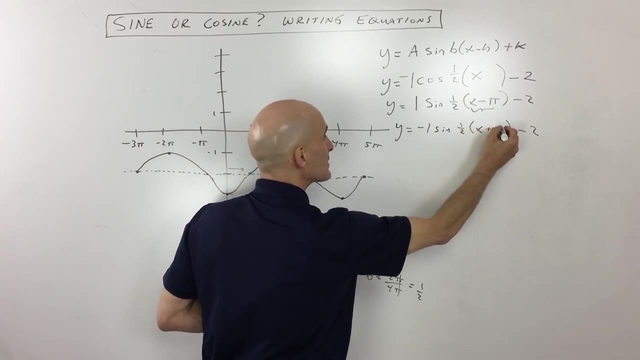 right, Okay, and it's going down, back up and like that. So that means now it's being shifted to the left pi, which means that this is actually going to be the opposite plus pi. Okay, remember, the one grouped with x has the opposite effect on the graph. And let's do, maybe. 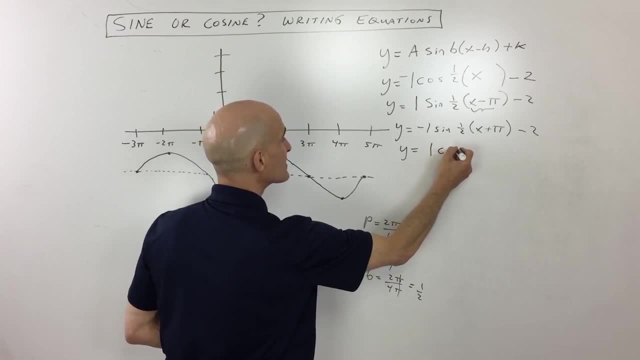 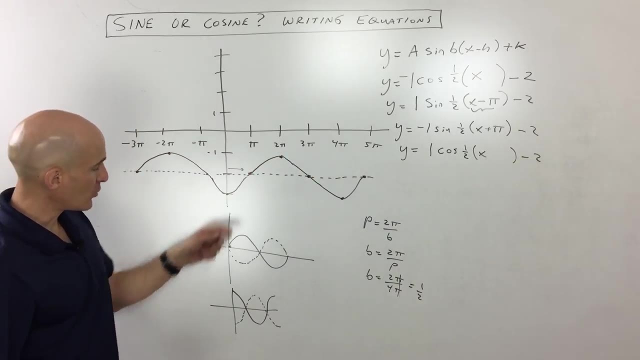 a cosine graph, and we'll just make this a positive one this time. The b value is the same, The vertical shift is the same. But now let's see. So if we do a positive cosine Now cosine, you can see, starts over here at the max. Okay, so we could either use this point here or we could.